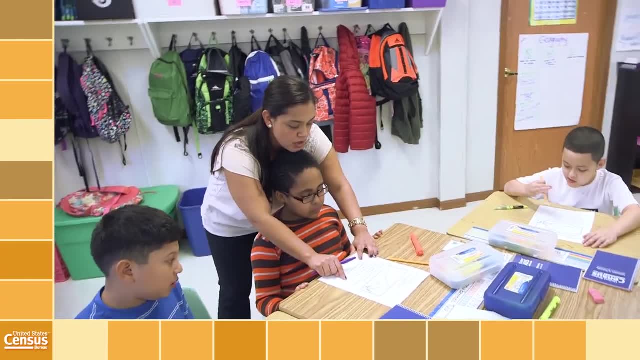 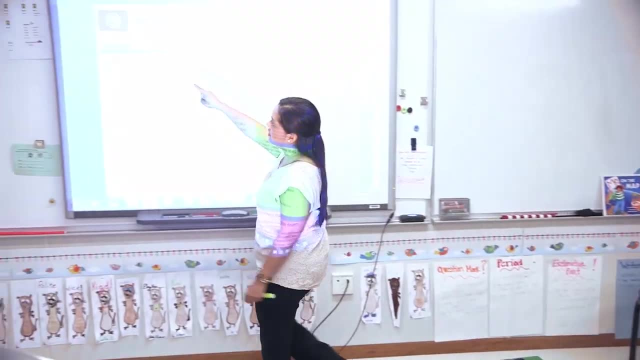 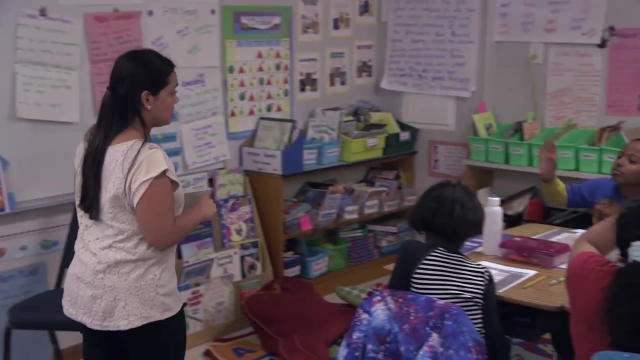 Statistics in Schools introduces students to the concept of data literacy, how they can turn numbers into useful information. So this population they're talking about is the number of people that live in Virginia. They go and they ask all these questions and so that's how we get all this information. 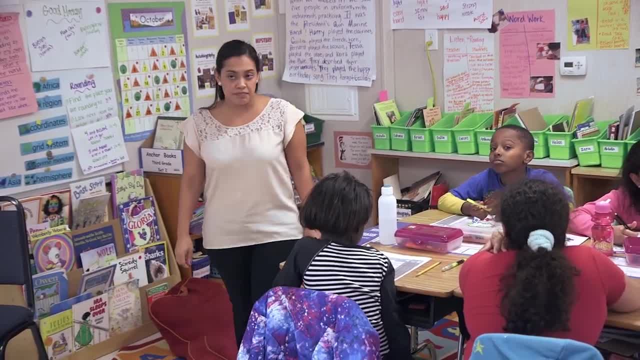 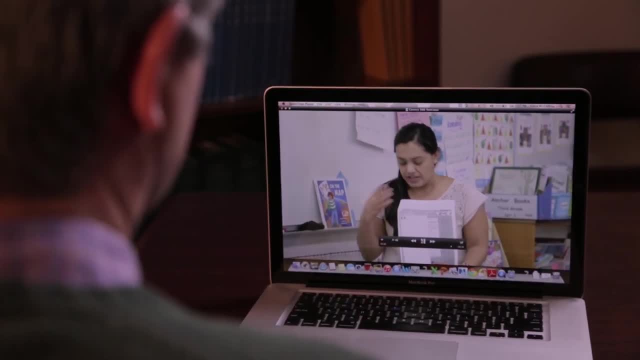 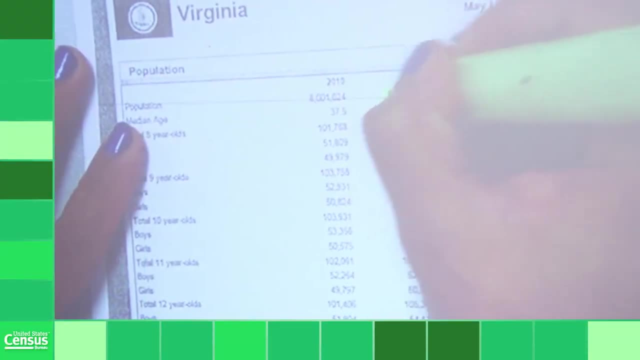 They mail it out. people fill out forms and that's how we know, thanks to the Census Bureau. What I liked about what I saw here was that the teacher was showing them a representation of where the data had come from, And I think it's great that students begin to see the data as something collected by real people under real-life circumstances and something that's happening every day around them. 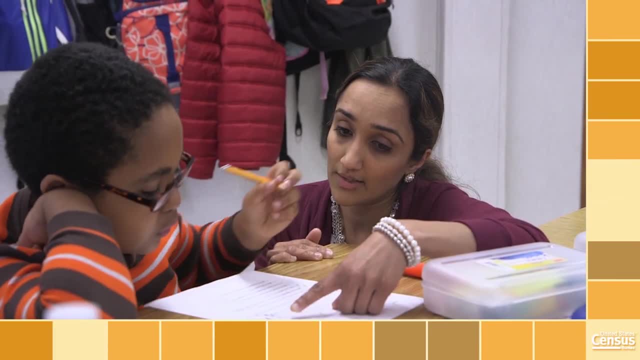 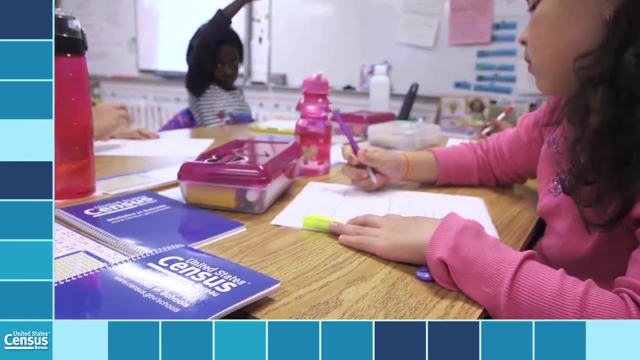 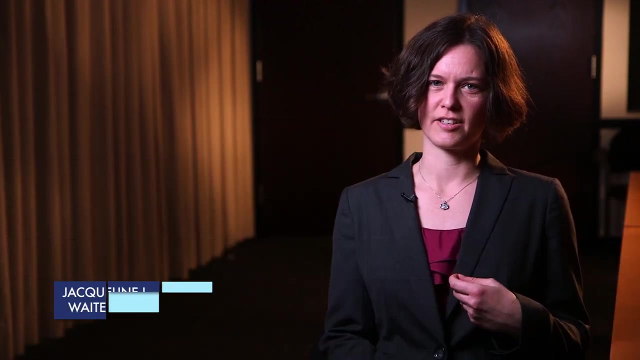 And that kind of drives home the relevance of it to their everyday lives. Statistics in Schools features maps that allow students to visualize changes in data over time. It's just such a natural fit between the data that the census is collecting and trying to understand what it looks like across space. 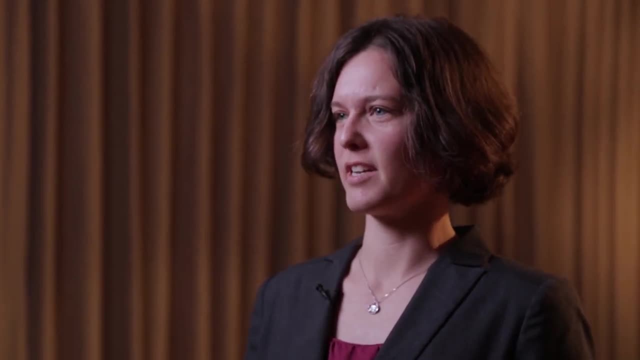 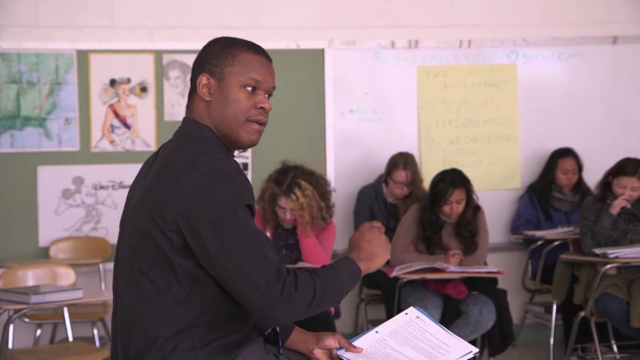 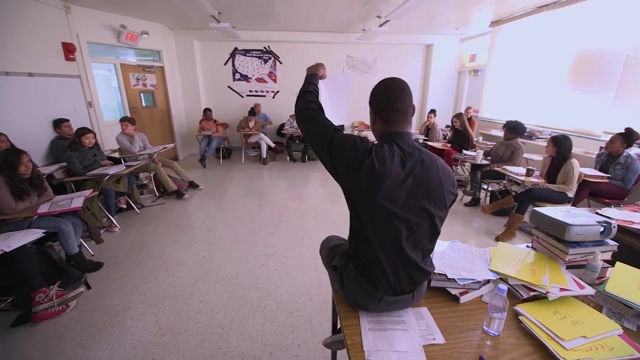 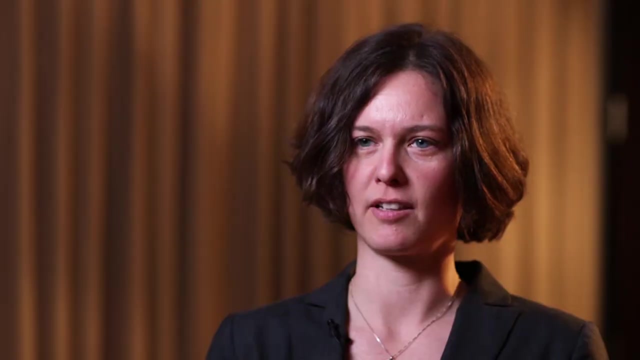 Why not add a map you know and why not really understand what maps can tell you? Look at the map right. Mark down things that you might be noticing. Mark down some interesting trends you might be seeing. The maps have really important information, not just about the data that it's showing, but it gives you a lot of insight into what policymakers were thinking about at the time. 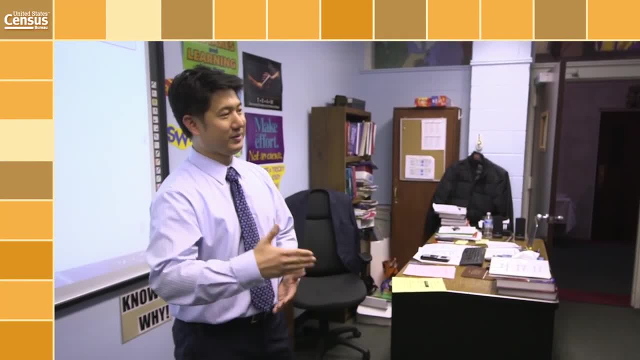 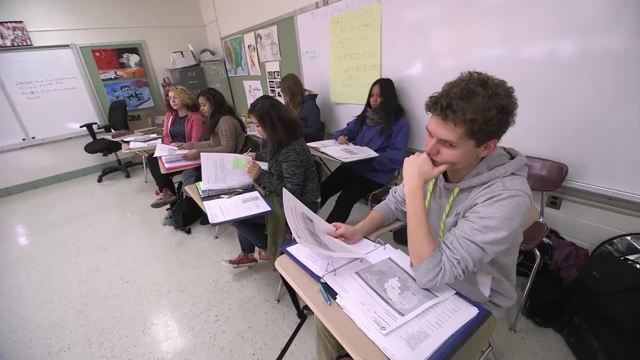 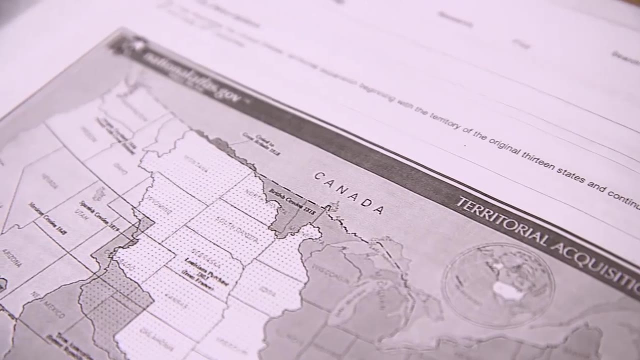 The interpretation of statistics lends itself to discussion and communication skills that all teachers want to incorporate in their classrooms. Do we have the exact number? Do we remember the exact number? How many? Do we remember Five thousand, Five thousand For a land to be considered a territory. 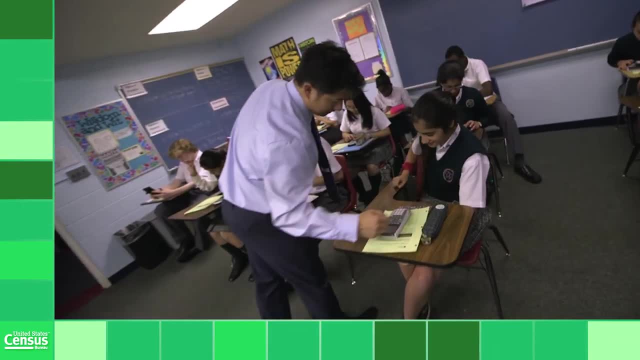 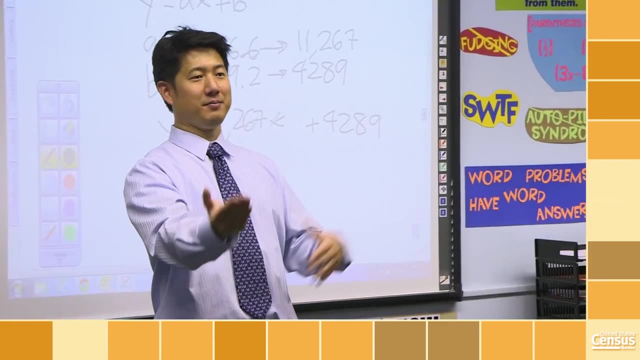 If you're teaching a history class, it's possible to teach it just as received wisdom, where I'm the teacher and I'm telling you what the facts are. But when we talk about analyzing data and looking for trends in the data, everyone can participate.